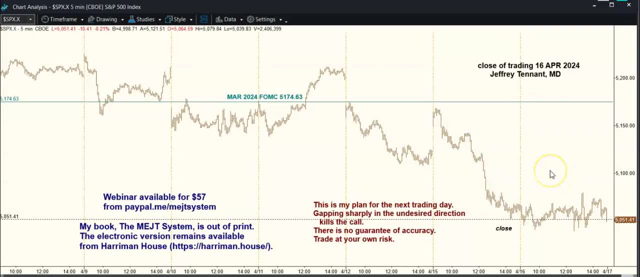 Well, we looked for the pattern: today with the early high, which is this, and tomorrow should also have the early high. We said this should either have a rally into the close or a straight line drop. Neither one of those things happened, but time doesn't run out until tomorrow's open. 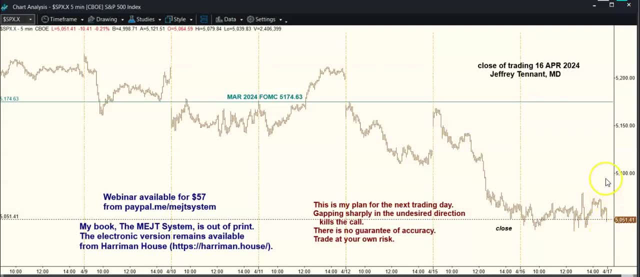 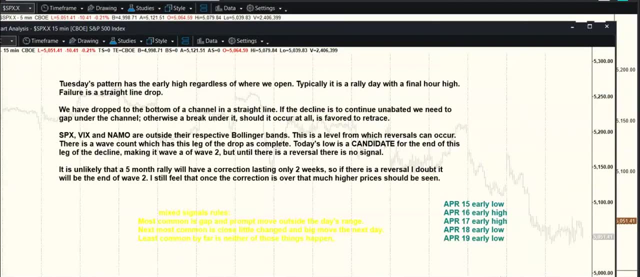 So either we should gap down smartly or gap up smartly at the open, and that would be the way the pattern works. It's a reminder of what we said We also had today as a candidate for the end of the leg of the decline. 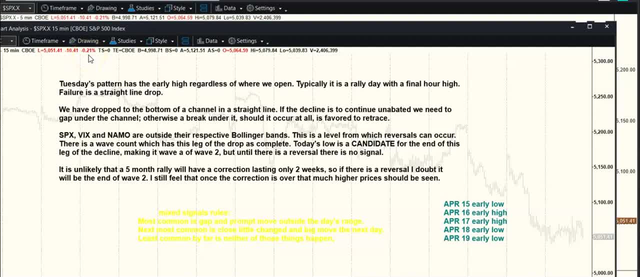 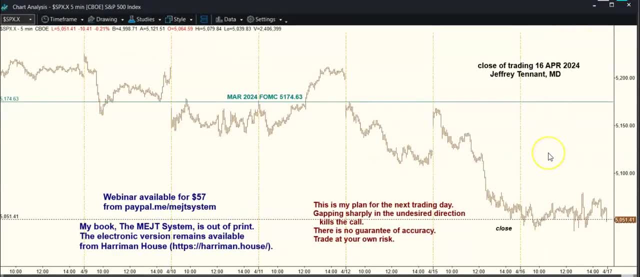 We closed a little change. I defined a little change. There's under a quarter of one percent. So I repeat my call: We have a candidate for the end of the low but there is really no signal for you to get the reversal And I think we'll find out early tomorrow. 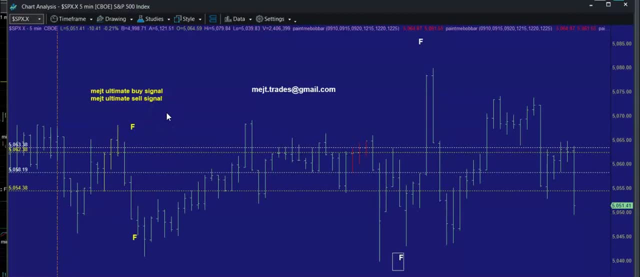 Early on we got an ultimate buy and an ultimate sell on the same pattern. So we traded higher, We traded lower. Neither one stuck. Usually when that happens it tells you the market's not going to do. The market does not want to make any progress for the next couple of hours. 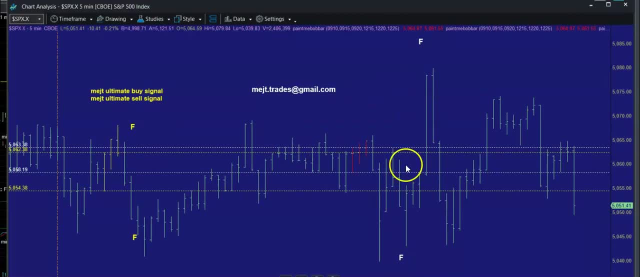 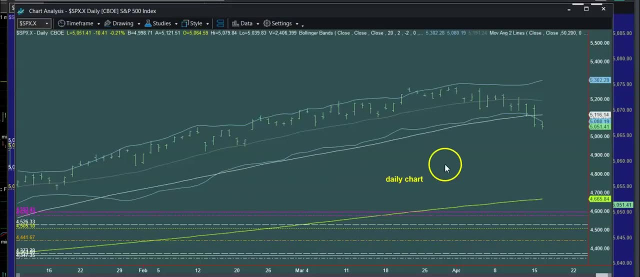 And we did In the afternoon. we traded lower, traded higher. System called them false moves and they've already retraced. There's the daily chart. Here's the Bollinger Band. One of the red flags for me is you have a bar completely under the lower band. 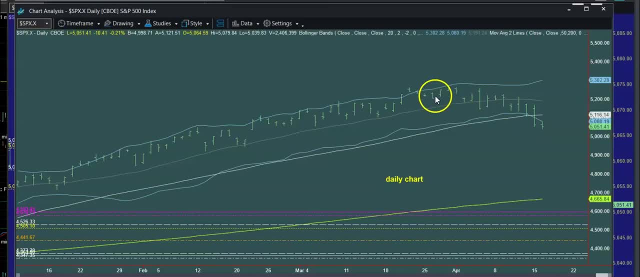 And the market often will do this prior to reversing. You can see here we have a bar completely over the Bollinger Band and then it was spent. So now we have a bar completely under the band. At least it's one of the possibilities. It's at least possible after this big drop. 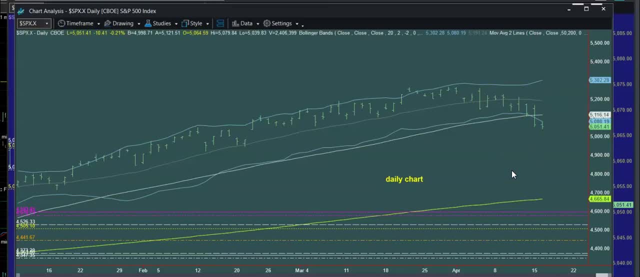 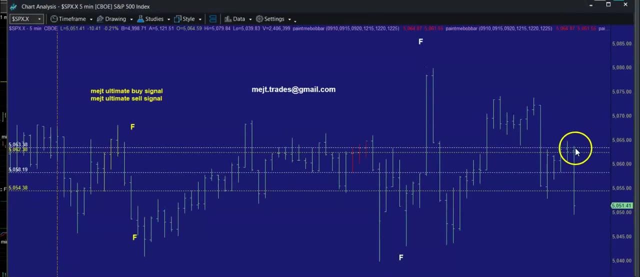 you're going to have a reversal tomorrow. Until it happens, you can't be sure, but at least it's one of the elements I look for. Another element is a wall into the close. These tend to be panic sells and they tend to reverse next day by capping up. 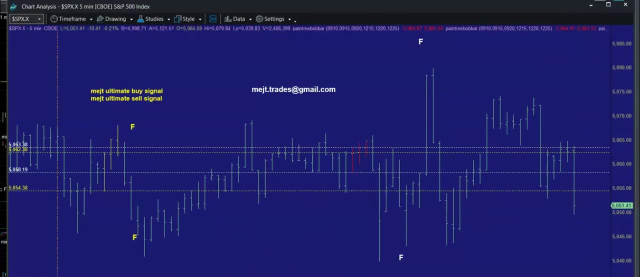 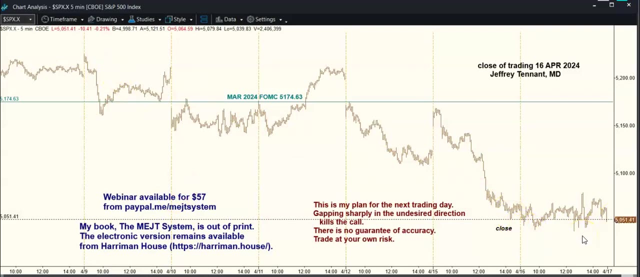 And you can see here that there's a lot of momentum in the low. It doesn't have to, but it happens often. Another thing is when you have a steep downtrend and you can't hold on to any of the day's lows. 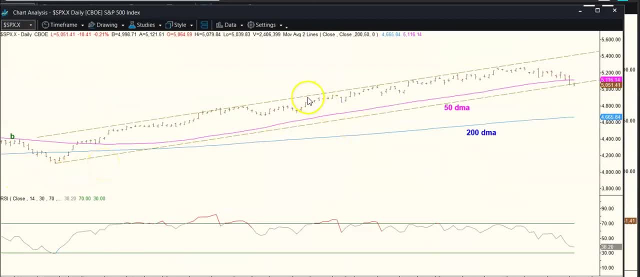 Now again, time doesn't run out until tomorrow morning. If we get down here, then you've done what you had to do. if you're a bear, Otherwise this is a candidate for churning at the low. Well, we said under this, like we went under the low, we went under the low and then we went under the low. 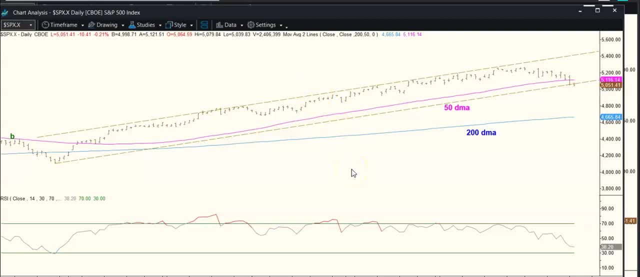 Well, we said we went under this, like we went under the low and then we went under the low. Well, we said we went under the low and then we went under the low. this channel, without the gap, it probably wouldn't stick. well, that's cutting it. 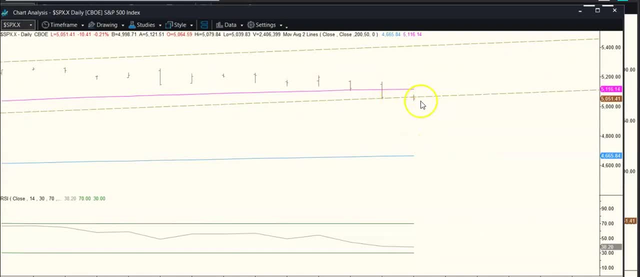 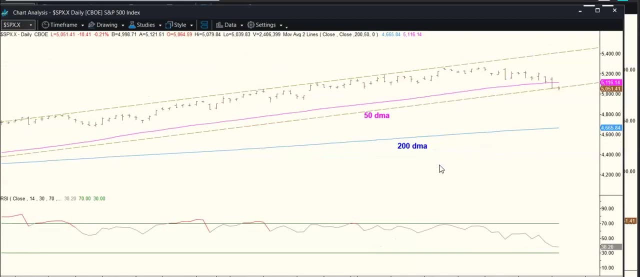 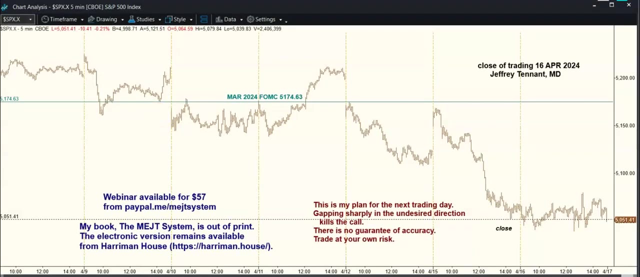 kind of close, but that's not a gap. so I think we're going to at least return to that channel, which doesn't have to be tomorrow. but again, it's not the kind of a clean break I anticipate if we're going to just keep on dropping well here. 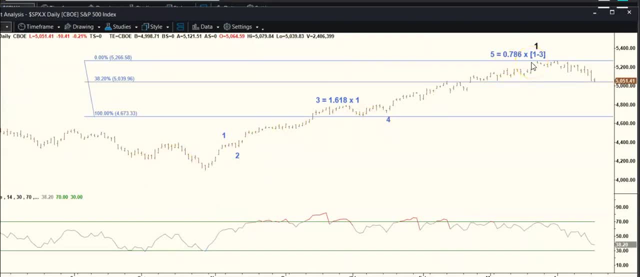 is the last rally leg and usually these things will correct 61.8%, but if it's extremely strong, the commonest place for a correction to stop is at the 38.2% and that's where we are. so it's again. I mean, if we get under it, then it didn't hold. 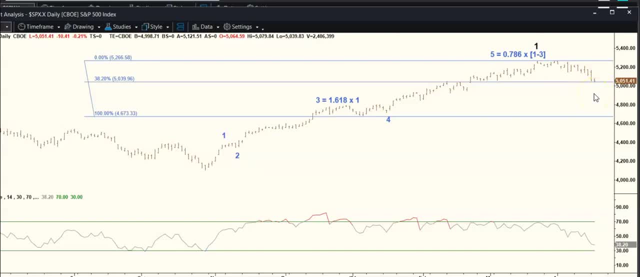 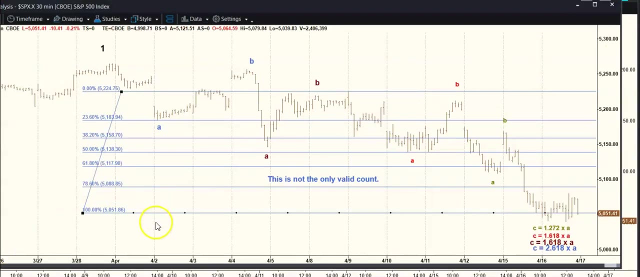 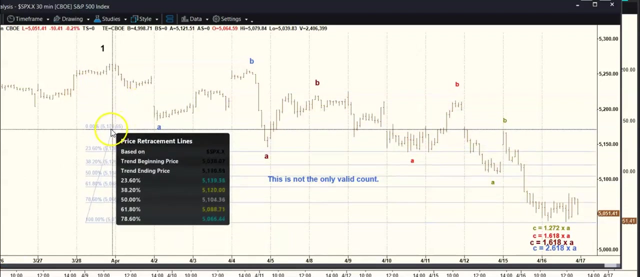 but it's one of the places, a common place for this leg to end, even though I don't think the whole declines over this leg- you as a candidate for this leg being over, we also have the kind of balance of the waves I look for. we made low. let's start with the smallest degree and work our 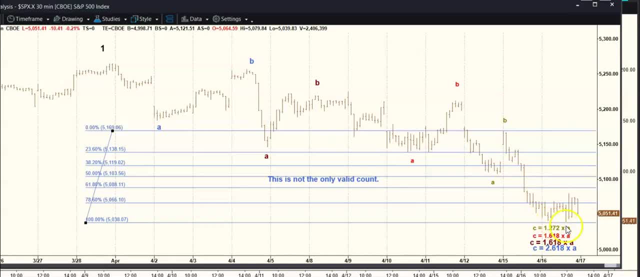 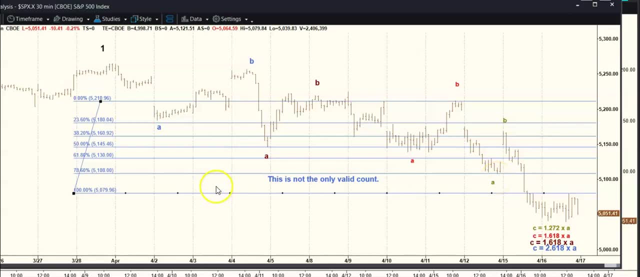 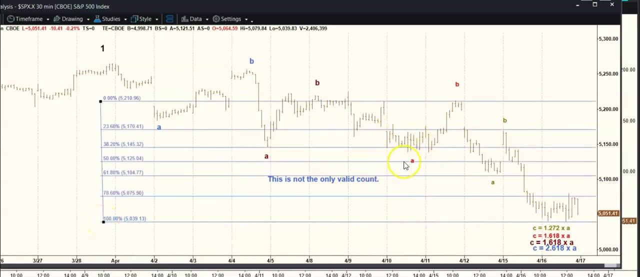 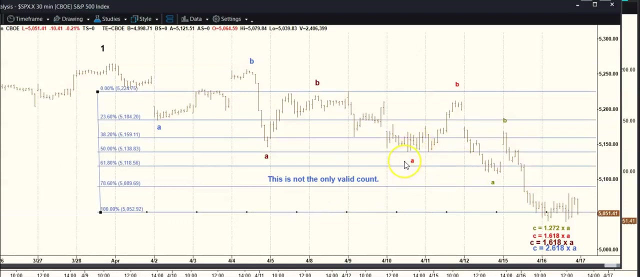 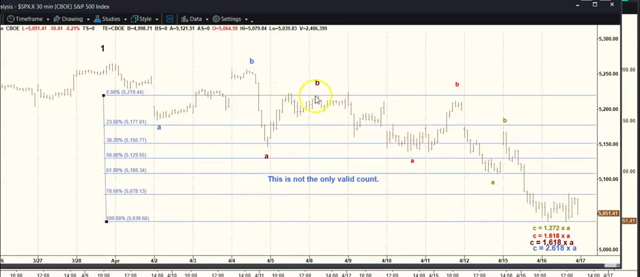 way up. here's wave gold. see to that low and there's fed balance with cool day. let's measure red sea from the top of wave of red a, not the origin but the top and the waves balance. now let's measure wave brown sea. that's the start of brown. 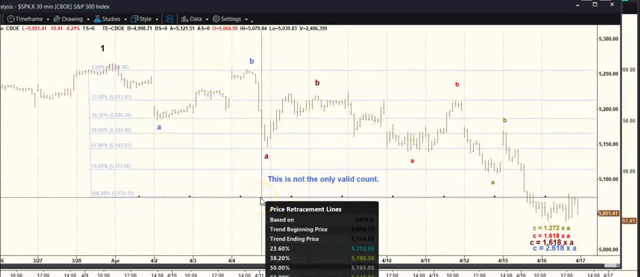 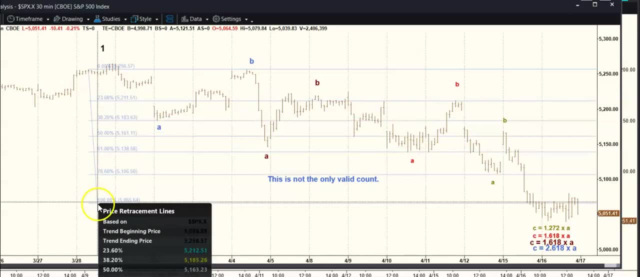 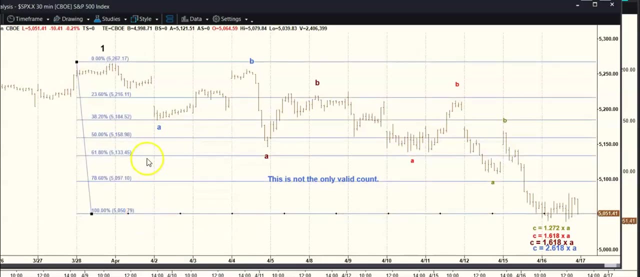 sea, and there, على the left, there's a wave on, the next wave on the right, out here, and we're going to draw out side the main had generals largest wave仆. The balance is this. one is, though, i'm going to They balance, and now let's look at the biggest way, which is pasegu know this. 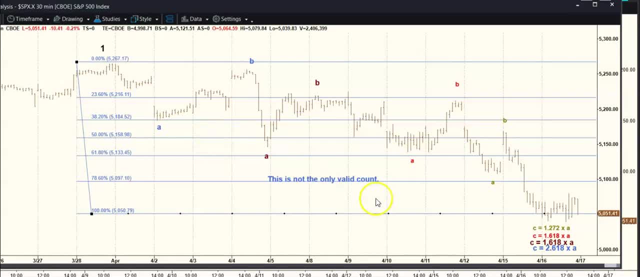 look at the biggest way, which is blue sea, and it's blue, a right there. now know this is a guarantee. it that's trying hold, but when you hit bottoms, I like to see balance of the waves like this, so this is a candidate. if they have holes, this first leg down could bail in this where blue waves can go. 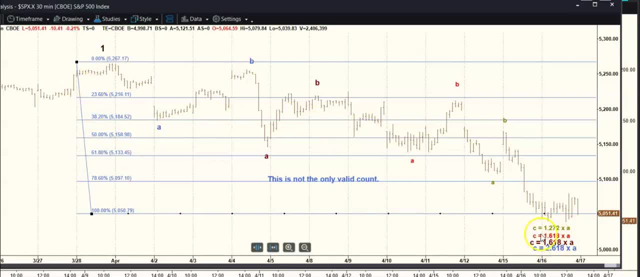 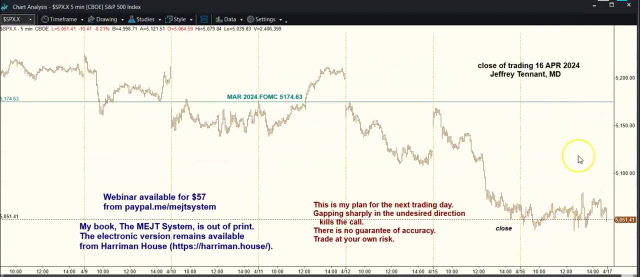 could well be over. we could have completed the blue abc because the fibs work, and if they don't work with all that evidence, then we're going to be gapping down and we'll know before the open. we gap up at the open, which i think is most likely, this abc down could be over. 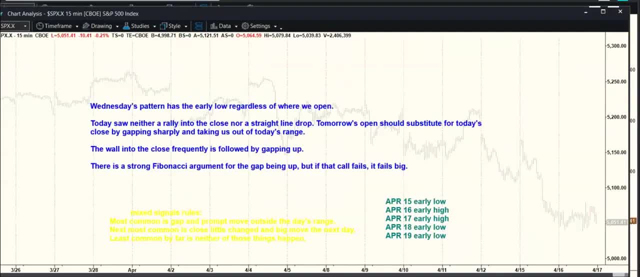 well, wednesday's pattern has nearly low. doesn't tell us where we open. today saw neither a rally into the close nor a straight line drop today's open. should tomorrow's open should substitute for today's close by gapping sharply and taking us out of today's range. the wall in the closes into the closes, frequently, not always, followed by gapping. 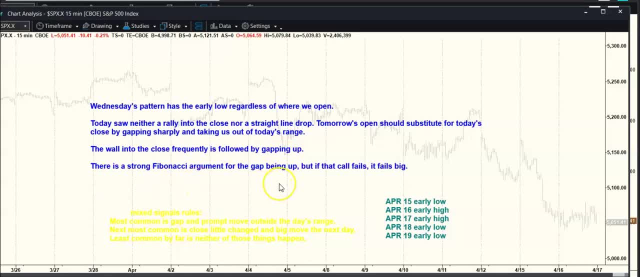 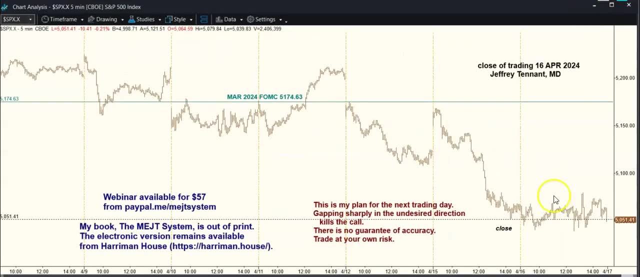 up and there's strong fibonacci argument for the gap being up. you just remember, if that call fails, it fails big big time, because when all these things are pointing to this slow holding and it doesn't hold, you could easily drop at least to the 61.8 retrace. 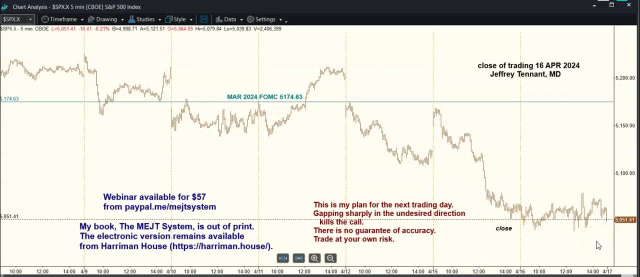 but for right now we have a good candidate for the end of the abc and blue down, which should lead to another abc, and blew up, which probably won't finish in a day. we'll have to see if we open up here, in which case that plays out as if we open up. 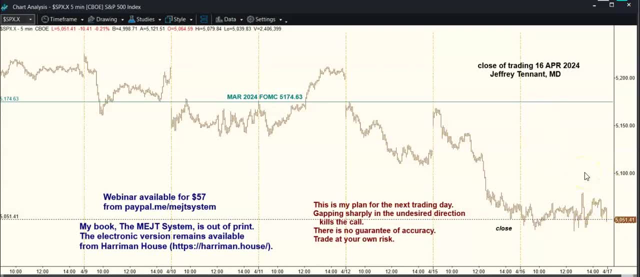 up down here. my eraser has to get taken out of storage, So tomorrow's pattern has the early high and that's today's call.